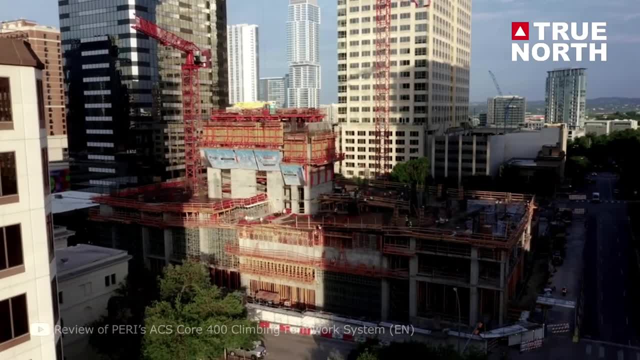 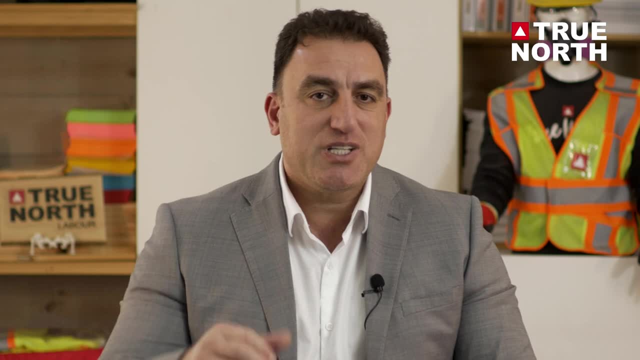 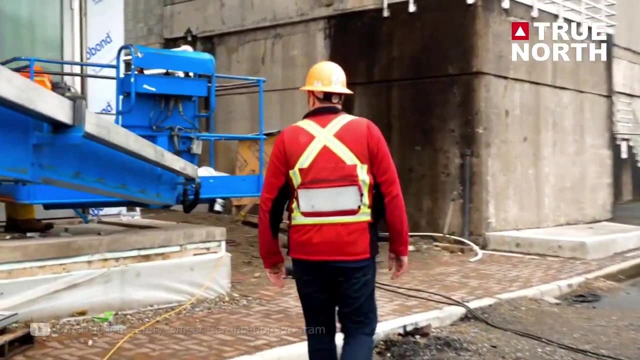 day-to-day operations. All of this comes with experience on the job for many of us. We found a way to expedite the knowledge part by using our 10-day rule for a CSO. 10-day rule is where CSO takes charge of the safety on site. 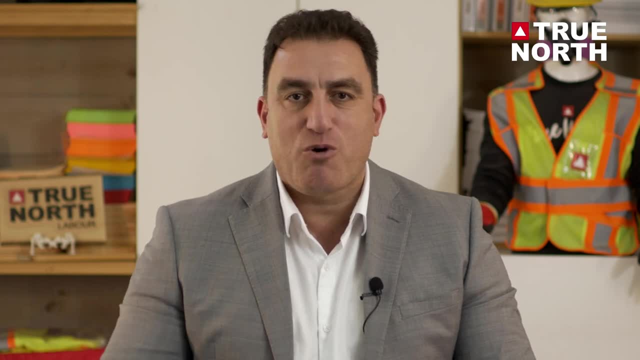 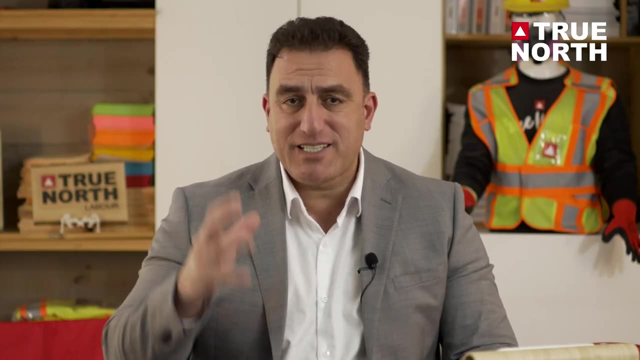 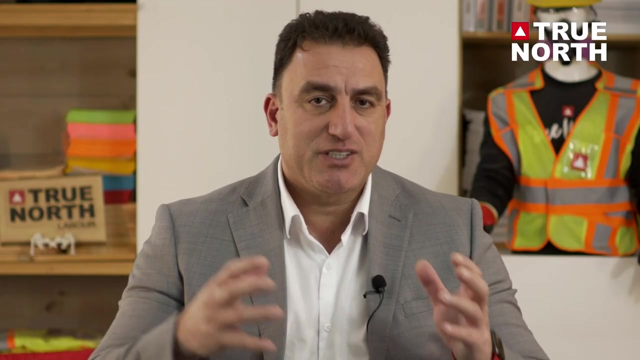 in a methodical way following a CSO roadmap. I will give you some examples of the first two days out of 10.. The role of a CSO is to identify, to inspect, then to describe and then to explain, Discuss, Find the person who is responsible for the task, equipment or an area. Then the CSO must. 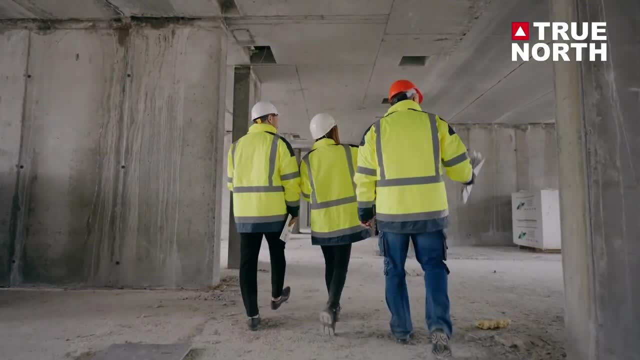 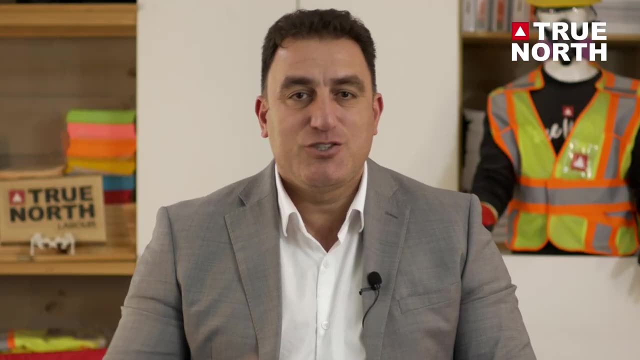 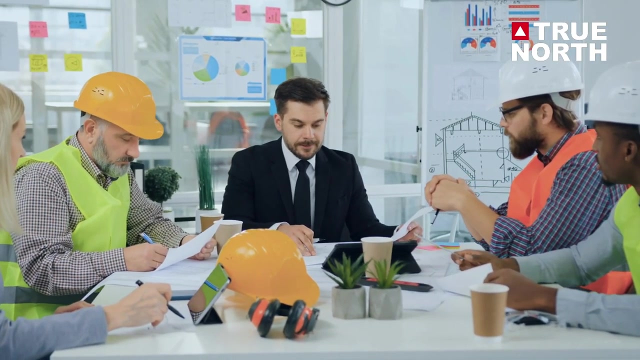 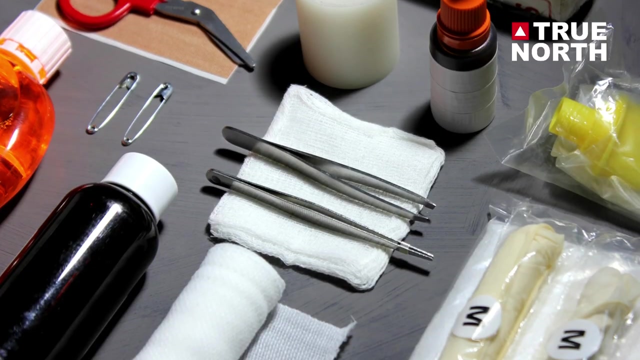 solve or delegate to a responsible person to correct or improve the subject matter. 10-day rule: day number one: Documentations, activities and inspections. A- Introduction to management staff and labor force for general contractor or subcontractor. B- Inspect and disinfect first aid room or first aid facility and take an inventory of supplies that you have. 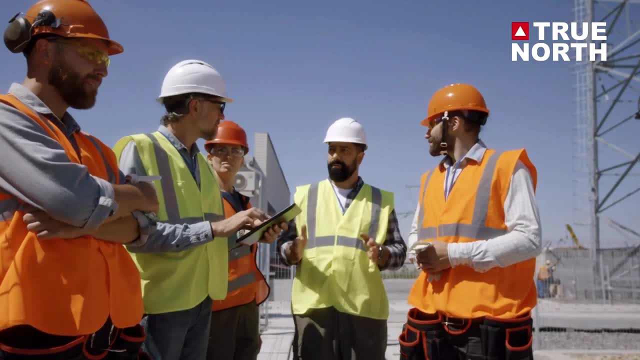 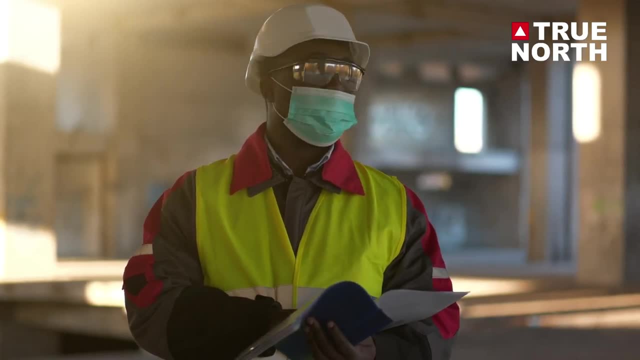 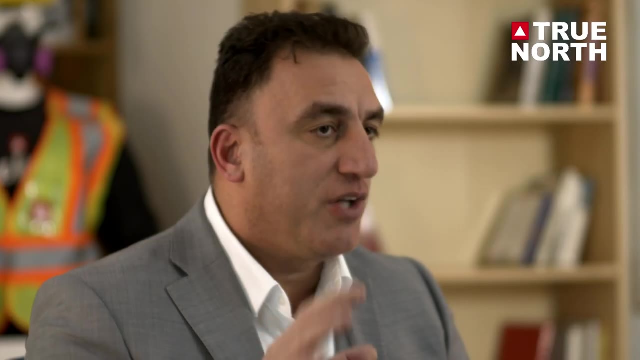 C Orientations, one or two a day. D- Two site inspections, one at 9 AM, one at 3 PM. E- Inspect emergency evacuation stations. F- Inspect the site, safety plan, rescue plan and a fire plan on the safety board by the trailers. 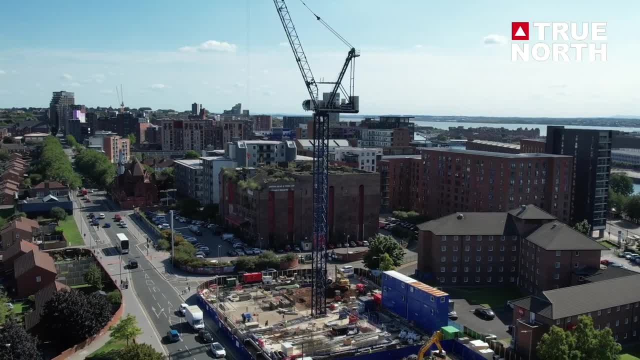 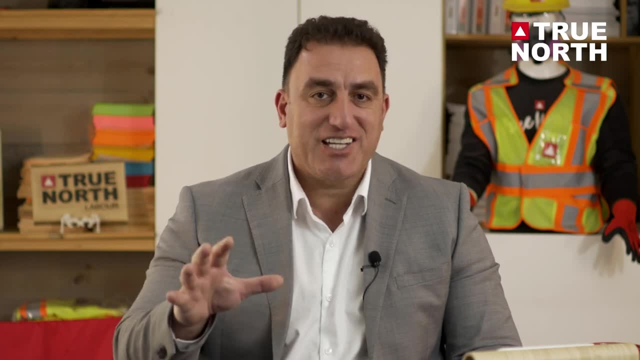 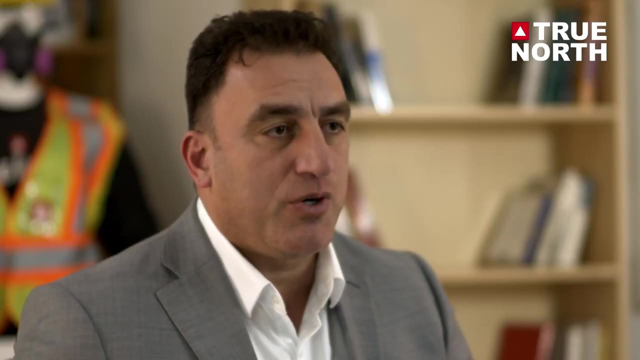 G, Site logistics and traffic control management. plan H- Noise by-law and work time hours. I Signage J. Do you need an inventory of things you might be missing? Fire extinguishers, air horns, eyewash bottles, K Daily sign-in sheets. 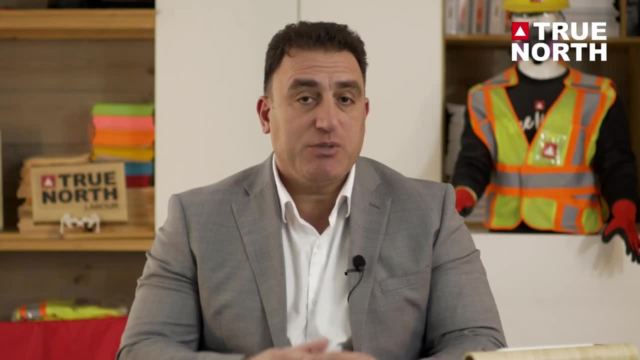 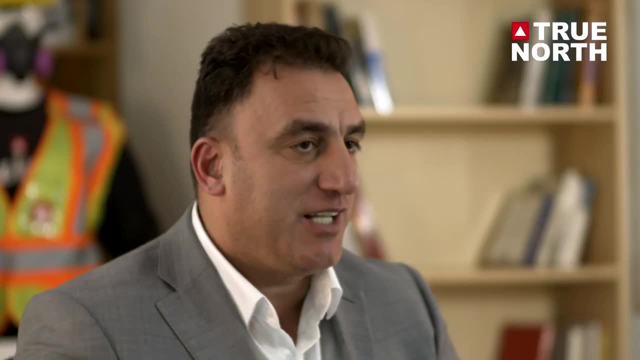 And L Radios. All of the above needs to be documented, looked after and also inspected. That is for day number 1 out of 10. for 10-day rule, Day number 2.. Documentations, site activities and inspections. 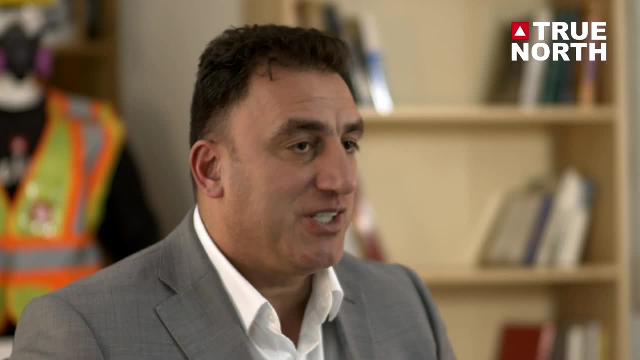 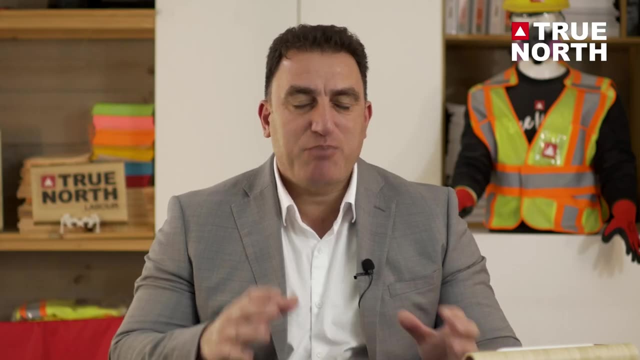 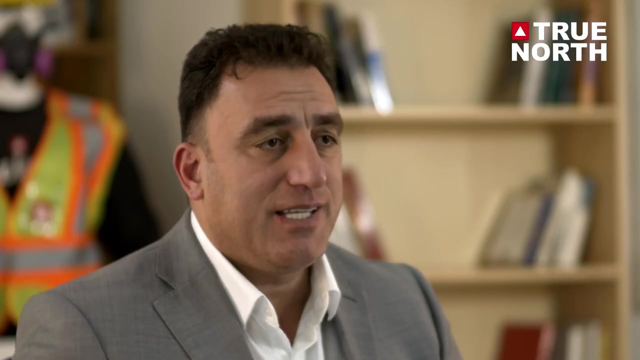 A- Public safety. We all know public safety is number 1. Traffic control management plan, Road and sidewalk housekeeping. B- Inspect and add safety signage and directional arrows on fences and trailers if it's missing. C- Inspect and ensure Safe access- egos.